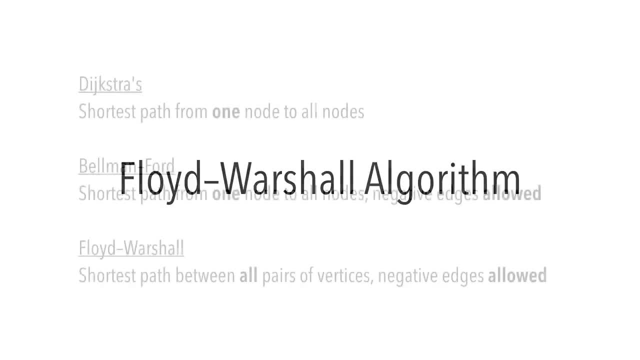 Today I'm going to teach you the Floyd-Warshall algorithm. First let's review its place among the other shortest path algorithms. Previously we learned that Dijkstra's provides the shortest path from one node to all nodes. Bellman-Ford is similar, except negative edges are allowed. Floyd-Warshall is different in that. 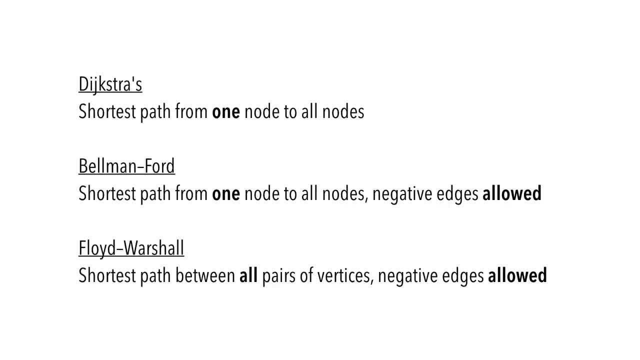 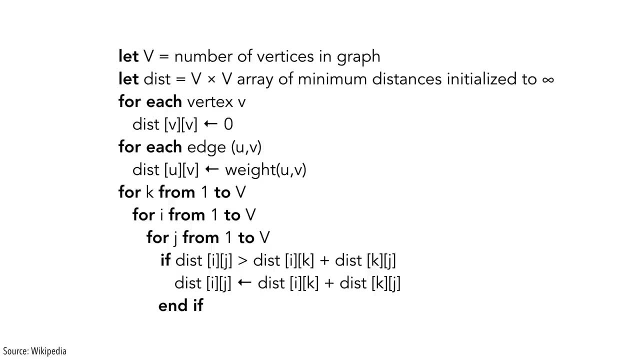 it discovers the shortest path between all pairs of vertices. Of course, negative cycles are not allowed in any of these algorithms. We'll start with the pseudocode, but don't be overwhelmed, We're going to walk through it step by step. First, we need a graph. 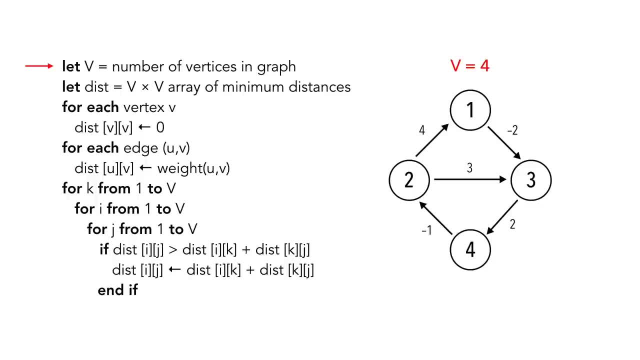 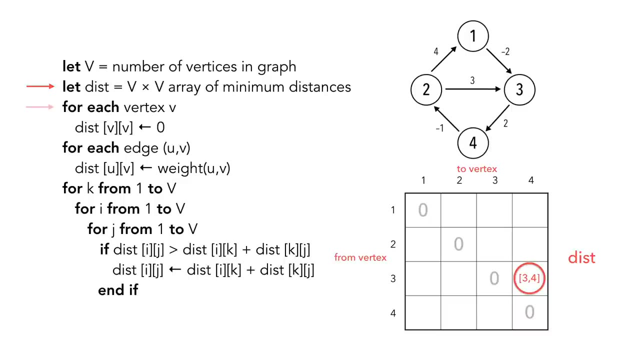 We'll use the one on the right. with four vertices, We create a distance array that keeps track of the shortest path between nodes. For example, row 3, column 4, will store the shortest path from node 3 to node 4.. Let's initialize each node's path. 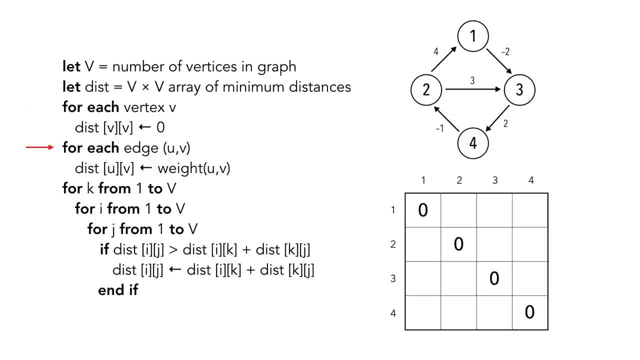 Our next step is to loop through the edges of our graph and fill in the table with the corresponding weight. We'll start with edge 1, 3,, which has a weight of negative 2, and add its value to our table. We loop through the remaining edges, adding their weights. 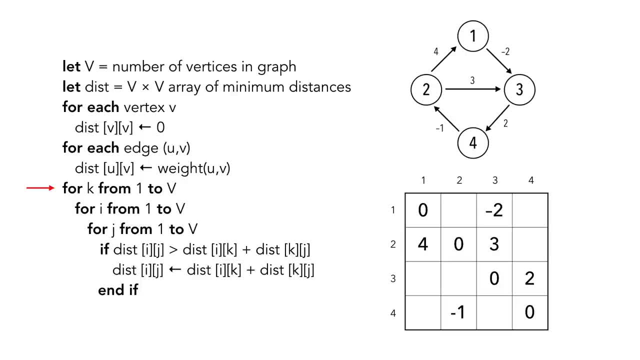 We're ready for the meat of the algorithm, the nested for loop. I'll hide most of the pseudocode, as our main concern is the if-conditioned and the three counter variables i, j and k. We start with them all equaling 1.. 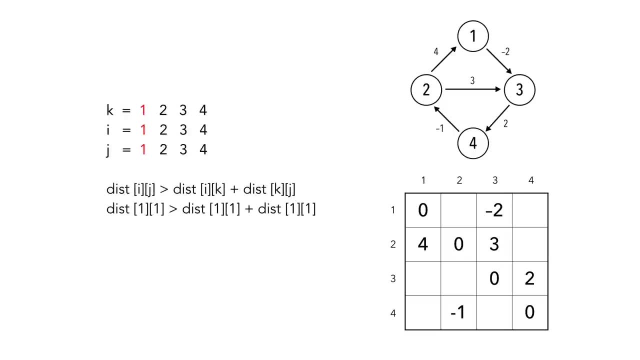 Let's fill in the corresponding values from our table. As you can see, the if-condition isn't met, so we don't update our table. Setting j to 2, we see the same result. We can see that our if-condition is not true and we don't make an update to the table. 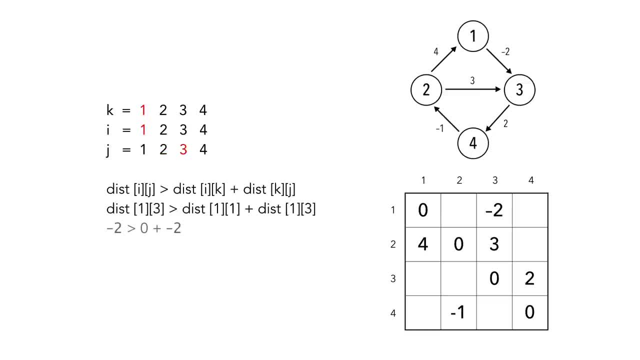 Likewise, when j is 3 and 4, our if-condition isn't true and we don't make an update to the table. This can be tedious, so let's skip ahead to an interesting iteration with k still 1, i equal to 2, and j equal to 3.. 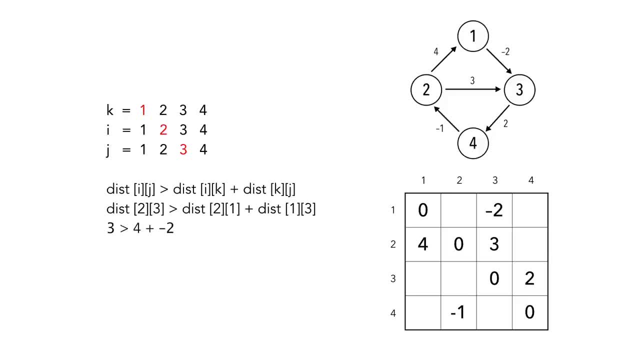 Plugging in the values, we see that this time our if-condition is met. therefore, we update the path from 2 to 3 with a smaller weight, which is 2.. Again, let's skip ahead to an interesting iteration, This time with k equal to 2, i equal to 4, and j equal to 1.. 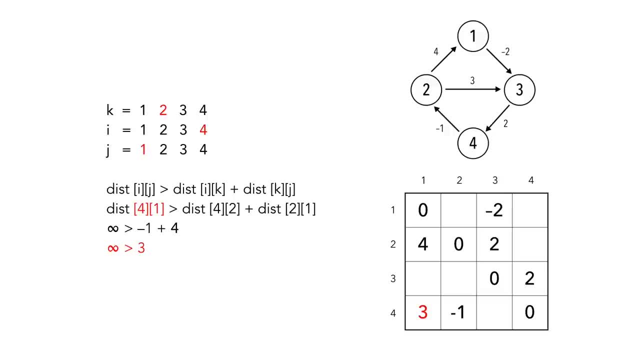 We found a new, shortest path from 4 to 1 with a weight of 3, so we update our table. By now I'm sure you see the picture. This is the pattern and flow of the nested for loop. I'll show you the rest of the algorithm without voiceover. 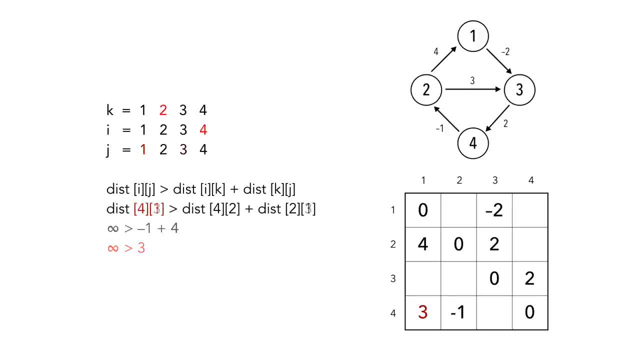 and I'll skip the iterations that have no effect on our table. Why is this going so slow? I just want you to see the pattern. that is always the same and the same as with the first iteration. If it's a general algorithm that I want to set to 0, then I just set a new knowledge options in place. 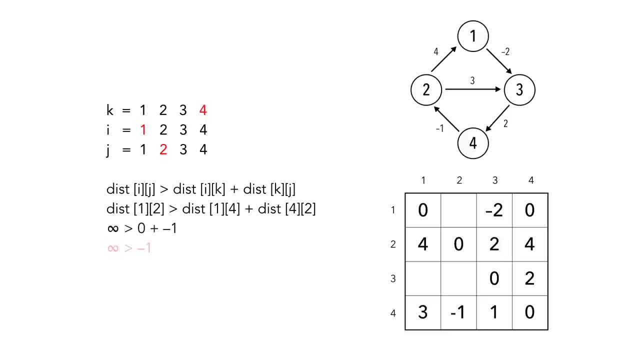 To see a change in this pattern. I can use the same new algorithm to see the change in the pattern or I can use the same algorithm to see the change in the pattern. So if I want to change something in the pattern to 0 or 0 to 1,, 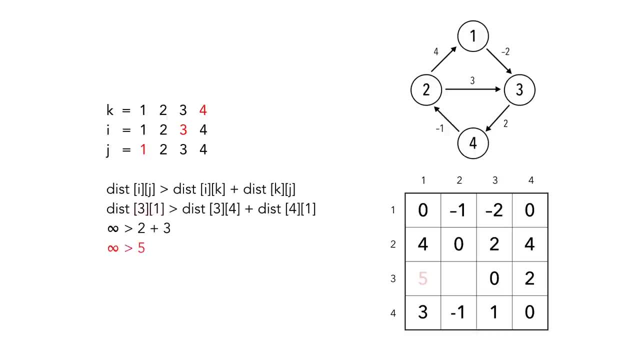 that's just my first step back and then go back to the first iteration and we connect the value to the first iteration. To do that, I'll just use the options that I've created in class 1.. So all we have to do now is select the new calculation. 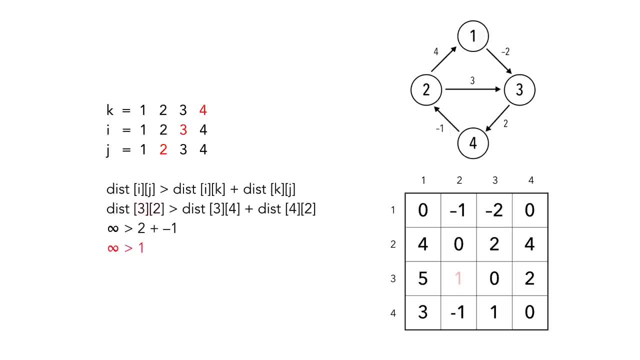 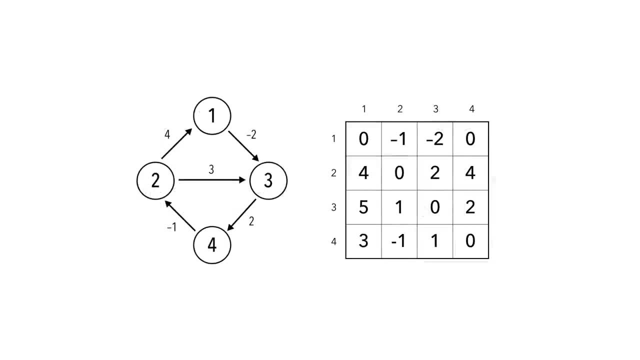 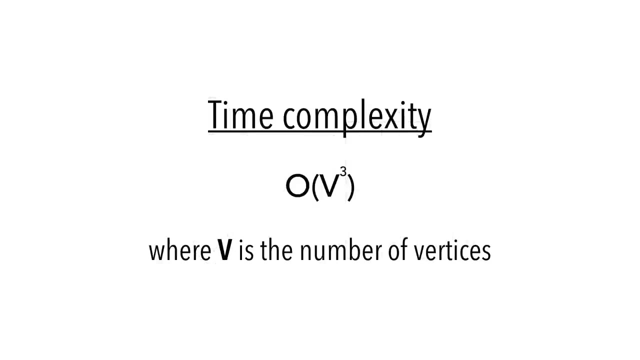 So if we want to change a parameter, which is the value of the error, This is the last iteration that affects our table. Here is our result: a table of shortest paths between all pairs of vertices. The time complexity of this algorithm is O, where v is the number of vertices. 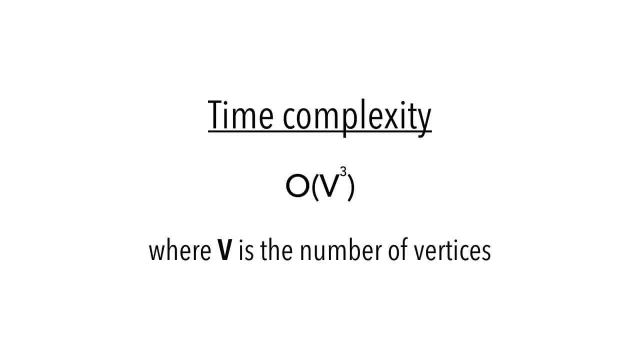 Because of this, I can't see anyone asking you to do this by hand, but hopefully this video improves your understanding of the algorithm and your ability to code it. As always, thanks for watching. There's a lot more coming, so please comment your suggestions below.